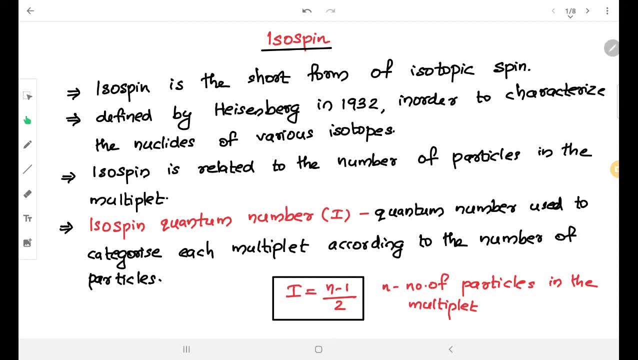 Then asked for strange particles, strangeness, quantum number. The next quantum number is isospin. So isospin is actually the short form of isotopic spin. This quantum number is defined by Werner Heisenberg in 1932 in order to characterize the nuclides of various isotopes. 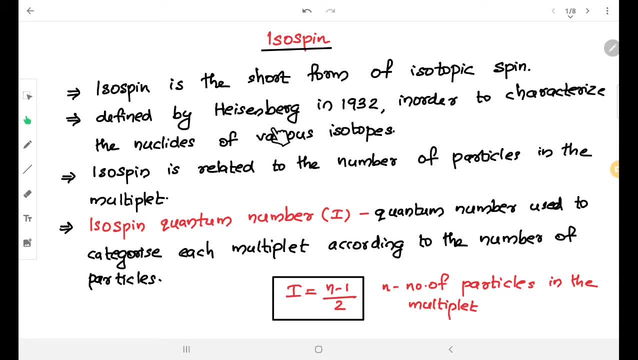 So here, according to Heisenberg, in the nucleons there are protons and neutrons, So nucleons composed of protons and neutrons. So Heisenberg defined this nucleon Nucleons as the two states of same particle. 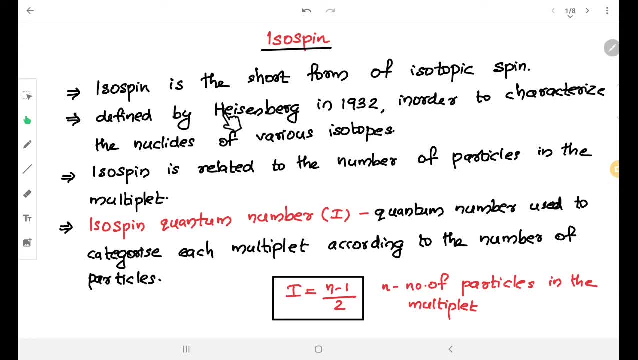 That means proton and neutron could be regarded as the two states of same particle nucleon. Similarly he grouped several other particles, So that group is known as multiplets. So in the last class we have discussed about multiplets. What are the characteristics of multiplets? 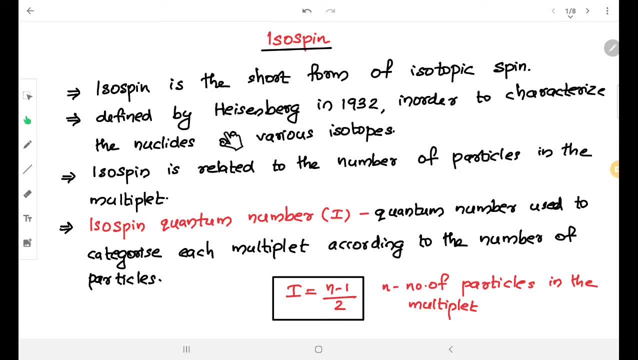 They have same spin, like that. So in the last class we have discussed about multiplets. So in the last class we have discussed about multiplets. So isospin is related to number of particles in the multiplet. 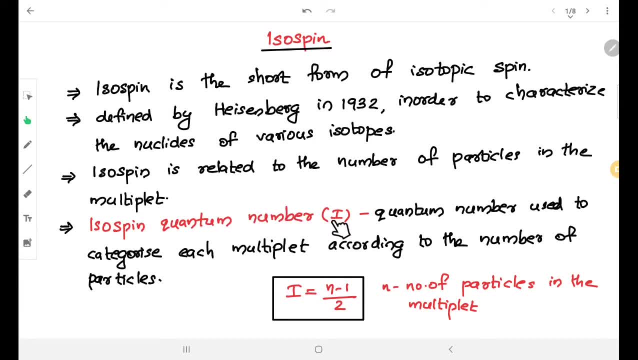 So isospin quantum number is denoted as capital letter I, So this is a quantum number used to categorize each multiplet according to the number of particles. According to the number of particles in a multiplet, this quantum number has a value. 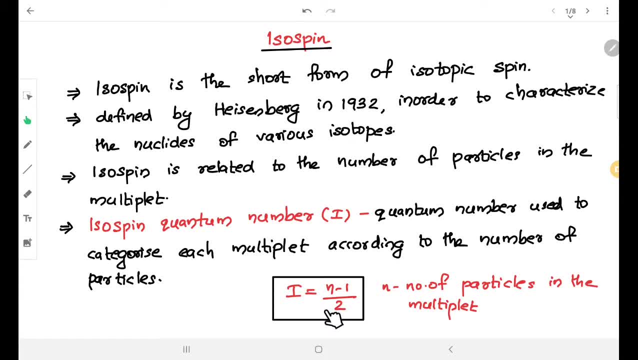 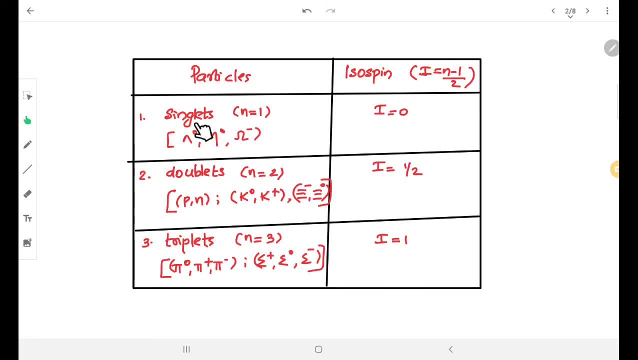 So we define I as I equal to N minus 1 by 2. Where N is the number of particles in the multiplet. For example, we can see singlets. We know that multiplets can be categorized as singlet, doublet and triplet. 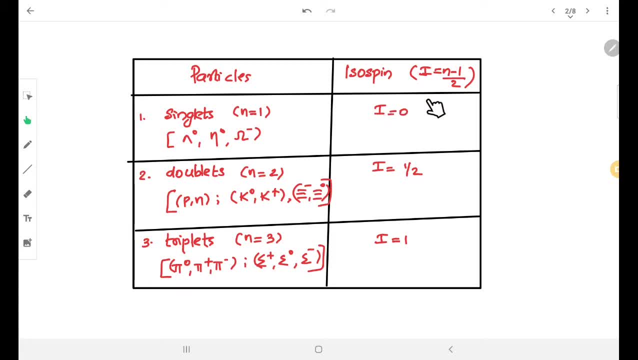 For singlet particles, isospin number is I equal to N minus 1 by 2.. So in the case of singlets, N equal to 1.. So I equal to 1 minus 1 by 2, that is 0.. 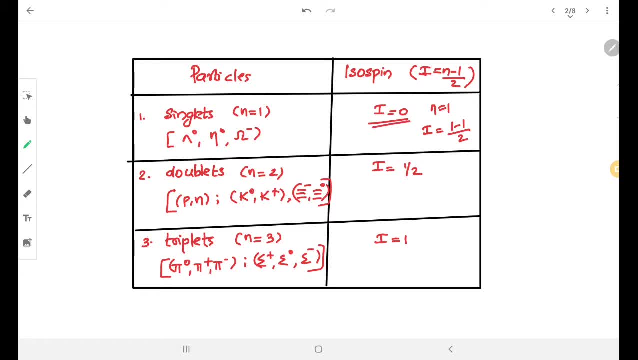 So I equal to 0 for singlets. Now for doublet. so singlets are lambda 0, eta 0 and omega minus. So singlets are lambda 0, eta 0 and omega minus. Now for doublet N, equal to 2.. 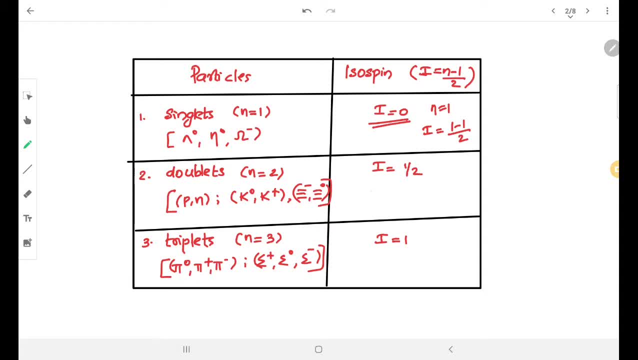 So when we put 2 in equation, I equal to N minus 1 by 2, we get I equal to half. So that means for all doublet isospin quantum number is half. So the doublet are nucleons, kions and psi hyperons. 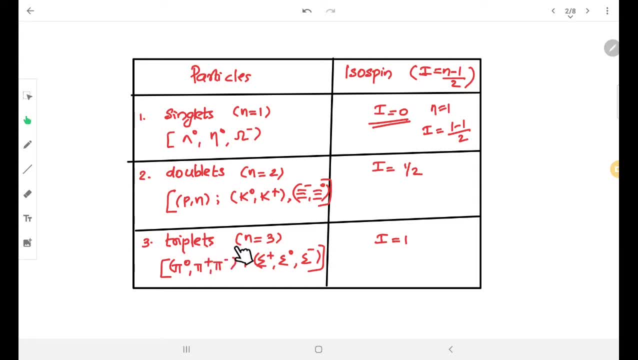 Next is triplets. In the triplets they have 3 members. So for this triplets the quantum number I equal to 1.. So the triplets include pions and sigma hyperons. So in this way we can categorize each multiplets and they can, each multiplet or each category of multiplets, have a particular isospin. 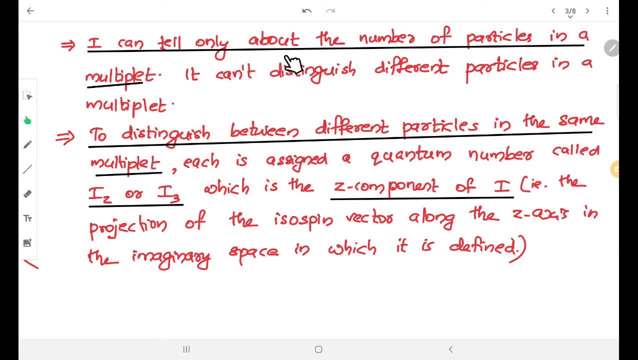 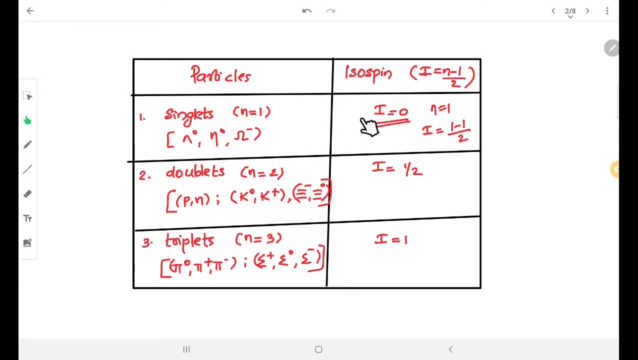 So what is the significance of isospin? Isospin can tell only about the number of particles in a multiplet. That means if it is a singlet we can clearly say that its isospin quantum number is 0.. 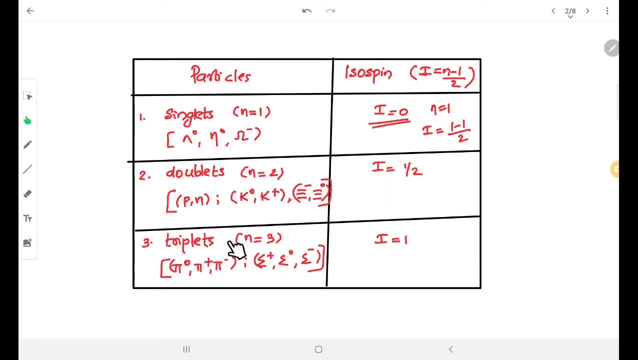 If it is a doublet, we can clearly say that its isospin quantum number is 0.. If it is a doublet, its isospin quantum number is half. Similarly, for triplets, its isospin quantum number is 1.. 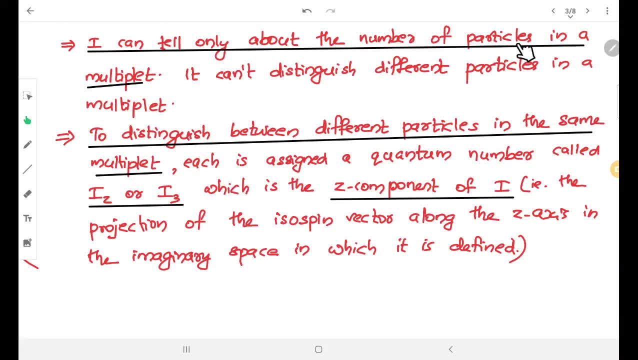 So isospin is a quantum number which tells us about the number of particles in a multiplet, But it cannot distinguish between different particles in the same multiplet. We cannot use this quantum number to distinguish between different particles in a single multiplet family. 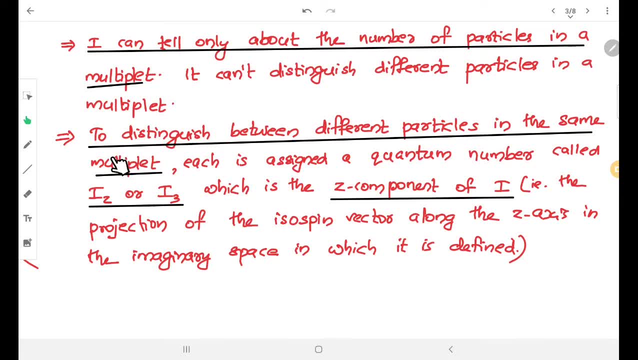 So for that we have designed a new quantum number for that property. So for distinguishing between different particles in the same multiplet, each multiplet is assigned a quantum number called IZ or I3.. IZ is denoted as I3.. 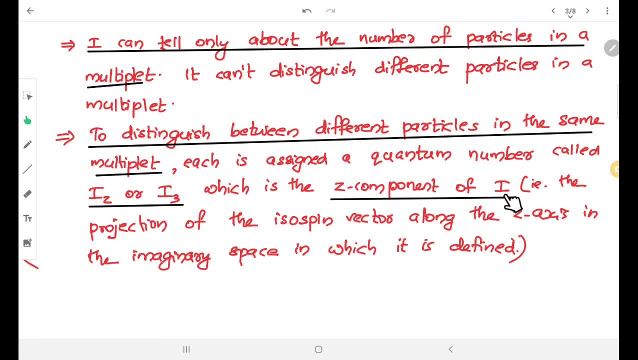 This is known as the Z component of I, That is, I is the isospin vector. The projection of the isospin vector to the Z axis is called IZ. So IZ is actually the projection of isospin vector along the Z axis in the imaginary space in which it is defined. 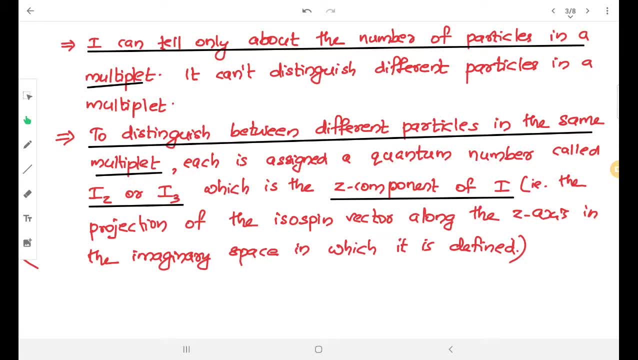 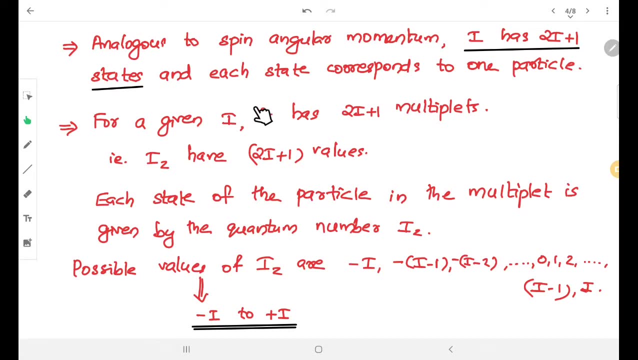 So to distinguish between a single multiplet family, we use the I as the distinguishing factor for a single multiplet family and we use the IZ as the distinguishing factor for a single multiplet of different particles in a single multiplet. Now the isospin quantum number is almost analogous to our spin angular momentum. 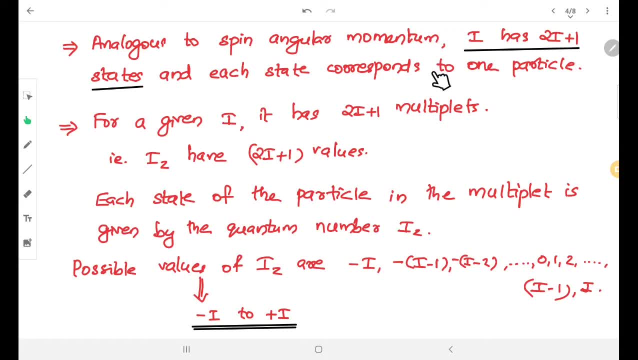 We have learned how to add spin to our spin angular momentum. Let us look at the possible orientations in that. Similarly, the isospin quantum number I has the same orientations, So there will be two. I plus one states in I: 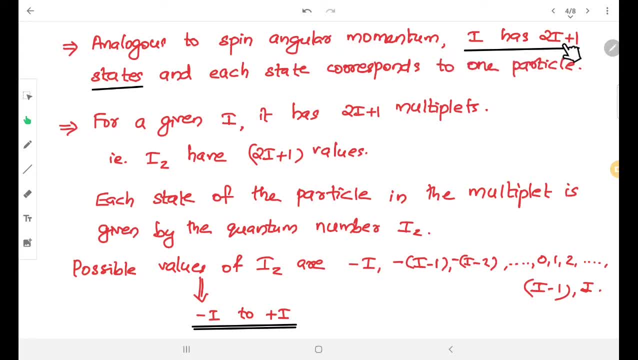 As we have learned, in angular momentum, just as there are two J plus one states, in angular momentum, there will be two I plus one states. in I, the isospin quantum number. Each state will be corresponding to each particle. So, to give an example, 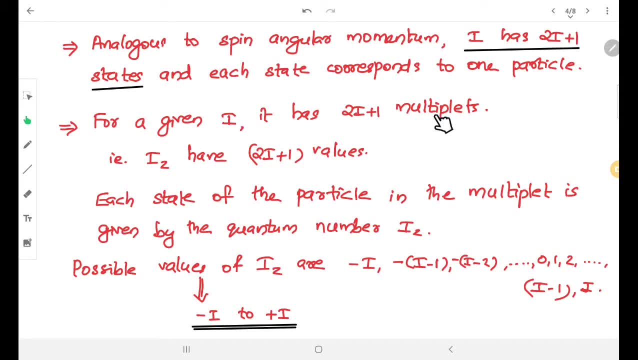 there will be two I plus one multiplets corresponding to a particular I, That is for IZ. there will be two I plus one values. Each state of the particle in the multiplet is given by the quantum number, IZ, That is, for a single multiplet family. the value of I will be the same. 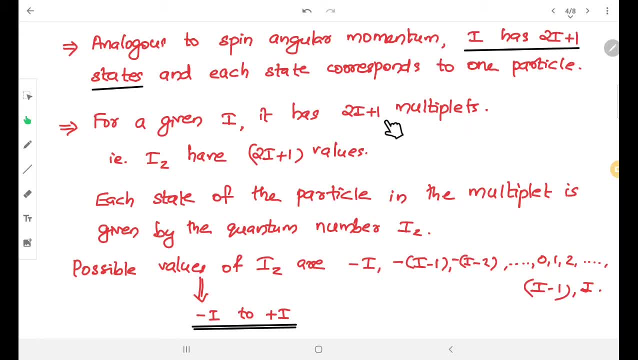 But within that multiple family, how many members will there be? There will be two I plus one multiplets, or two I plus one members. Each member will have a value of IZ. Now we can distinguish each member. So where does the possible values of IZ vary? 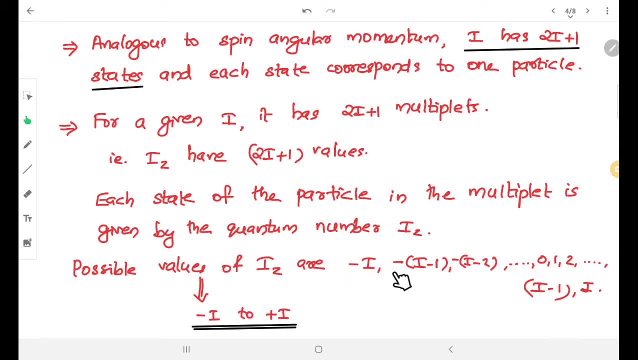 It varies according to our spin orientation: Minus I to plus I. The difference in magnitude of unity, That is, when minus I is given. it varies according to one unit difference: Minus I, minus of I, minus one, minus of I, minus two, etc. 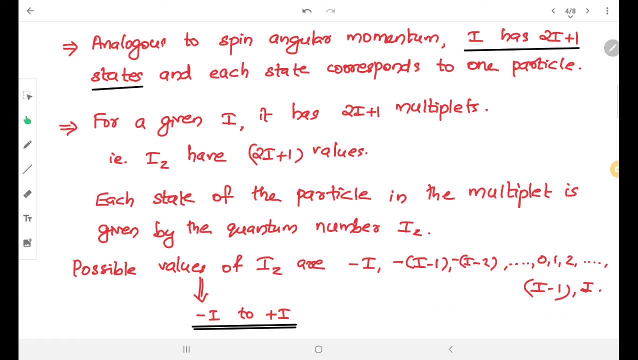 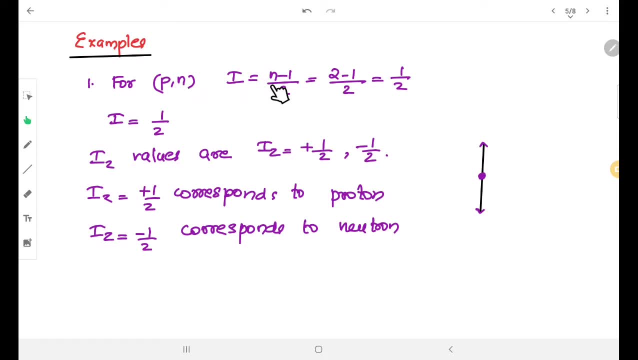 Zero One, two, etc. I minus one. I. Now we can understand by looking at the example. Let us take the nucleon family. In the nucleon family, since I is equal to minus one by two, N2,. 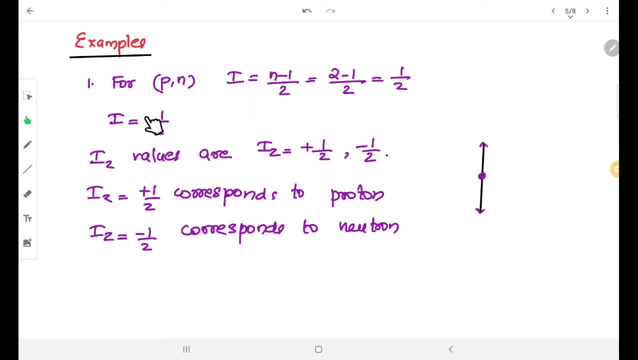 we get I equal to half. So for this family the isospin quantum number is half. But where does the IZ value range from? It ranges from minus I to plus I. Minus I means minus half to plus half. 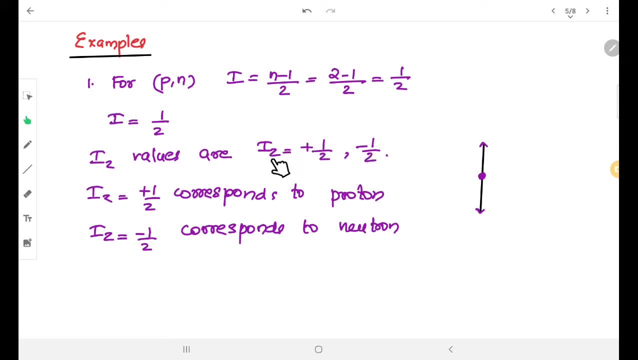 That is the value of IZ. So there are two possible values of IZ: IZ equal to plus half and IZ equal to minus half. When IZ equal to plus half, the proton, the particle with the highest charge, state. 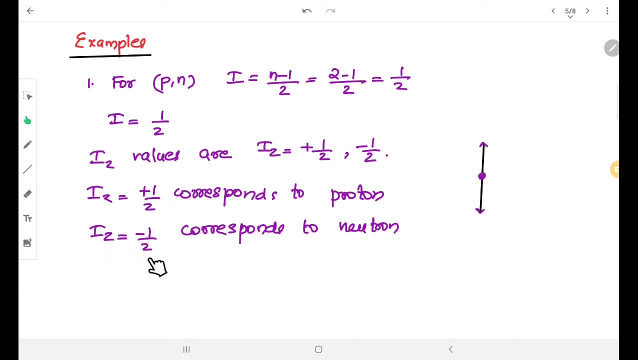 can be positive for IZ. IZ equal to minus half corresponds to neutron, That is, in this direction. it will be proton. The IZ value of proton is plus half In the upward direction, The neutron which is oriented downwards. 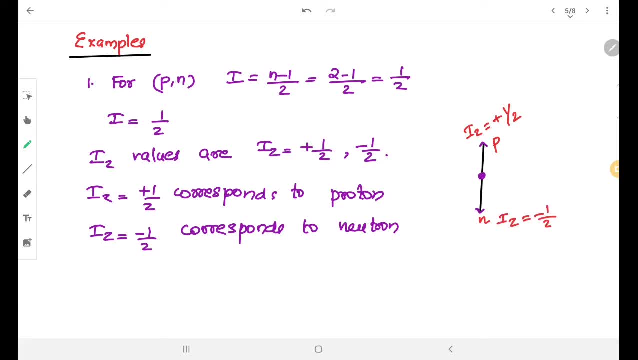 its IZ value is minus half. Now let us introduce a doublet like this: Si minus and Si zero. The I value of Si minus and Si zero family is half, Because N2 is the same. So for the Si family and the nucleon family, 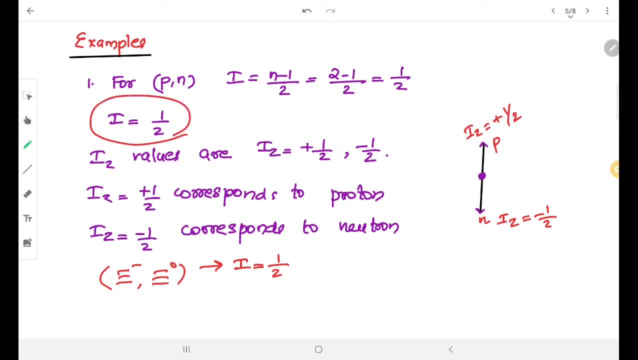 the isospin quantum number is the same, But how does the IZ value come? The IZ value, as we said earlier, has two possible values: Plus half and minus half. In Si minus and Si zero, the charge state is more than zero. 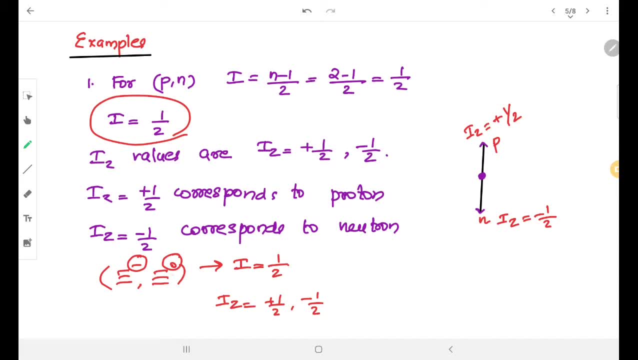 The negative value comes after zero. So the charge state is more than Si zero. So that is the upward direction. So in the upward direction, Si zero and in the downward direction it will be Si minus. Okay, So the corresponding IZ value of Si zero. 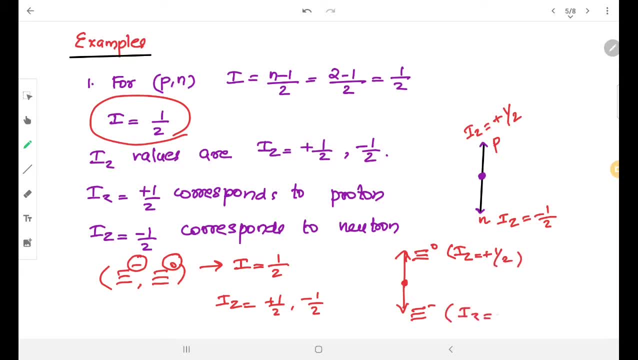 plus half and the corresponding IZ value of Si minus is minus half. Okay, In this way we can distinguish each doublet, each particle. So if the value of IZ is upward, if the IZ is in the upward direction, 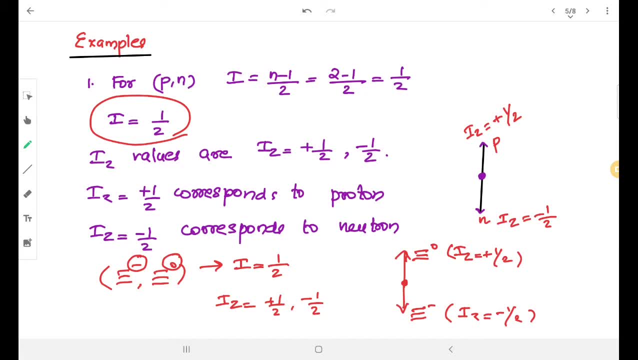 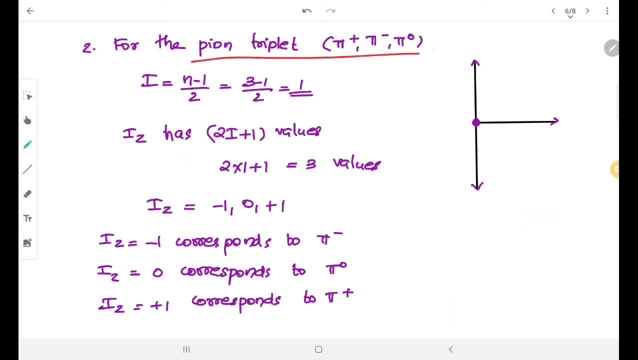 that corresponds to Si zero. So to identify the members of the Si family, what can we use? We can use the quantum number, IZ. Similarly, we can see a triplet here: Pi on triplet. Pi on triplet, The value of I is one. 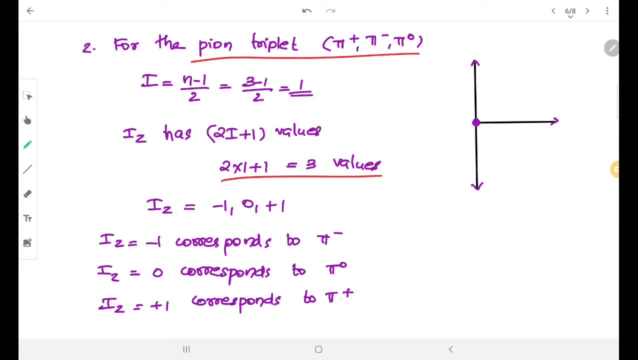 So how many possible values will be there in IZ? Two I plus one, That is two into one plus three. Two into one plus one, That is three values. What are the possible values? Minus one, zero one. 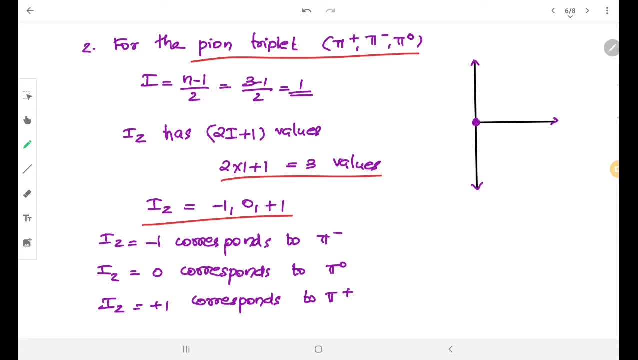 So in this Pi plus, Pi zero, Pi minus, the charge state is more than Pi plus. Then, after Pi plus, the next charge state is Pi zero. The most negative charge state is more than Pi minus. So which is the charge state? 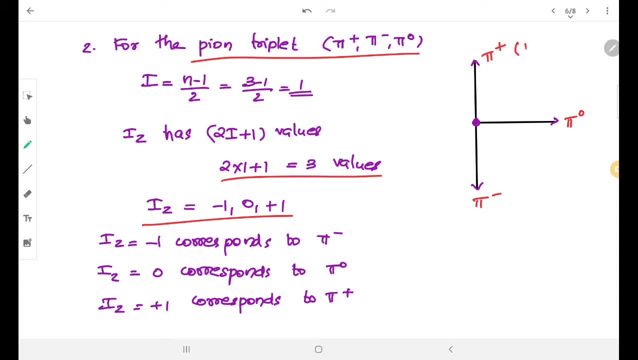 If Pi is not corresponding to Pi, the IZ has a positive value. If Pi plus is corresponding to Pi, the IZ value is plus one. If Pi zero is corresponding to Pi, the IZ value is zero, And if Pi minus is corresponding to Pi, 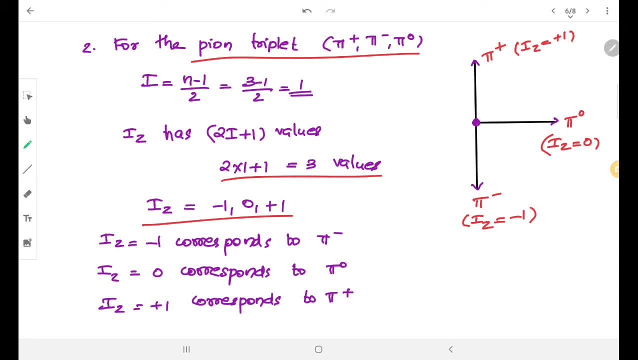 the IZ value is minus one. So in this way we can orient Pi ions in an imaginary space. Okay, So the projection of the isosceles is what we can distinguish between these three particles. An isosceles. 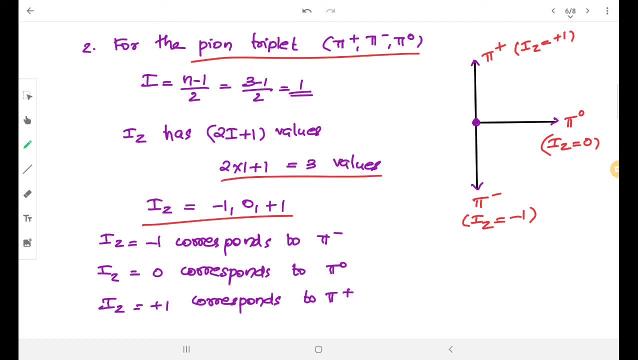 an isosceles quantum number and an isosceles triplet family are denoted, In that the isosceles Z component is used to distinguish each particle. Okay, Next, an important conservation law of the isosceles and the IZ. 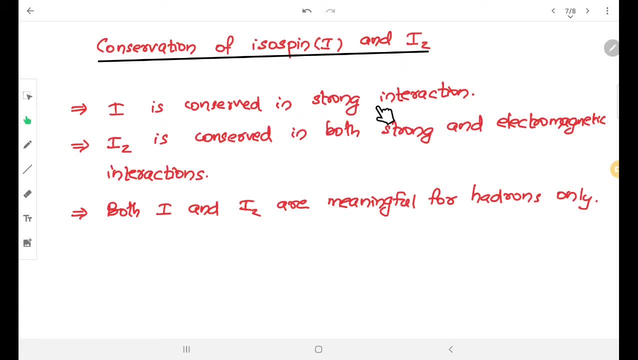 Conservation of isosceles and IZ. I is conserved in strong interactions, But IZ is conserved in both strong and electromagnetic interactions. So I and IZ are conserved in particular interactions. I is conserved in strong interactions. 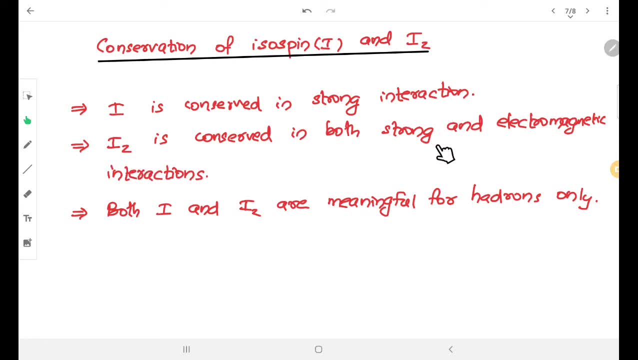 And IZ is conserved in both strong and electromagnetic interactions. These I and IZ values are applicable only for hadrons Because, as we said, multiplets, singlet, doublet, triplet are valid only for baryons and mesons. 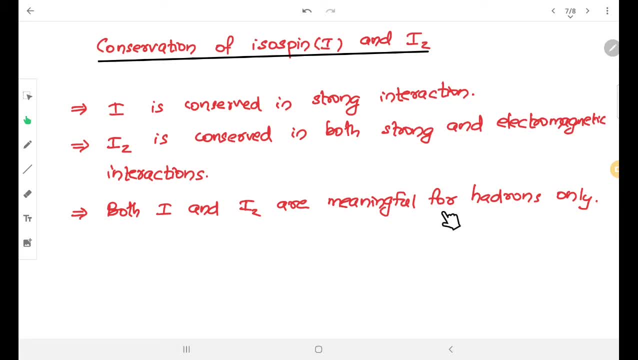 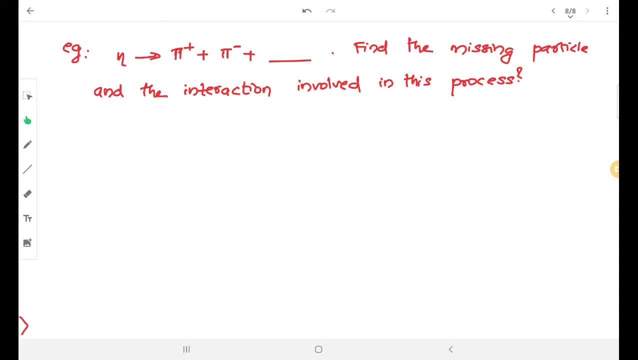 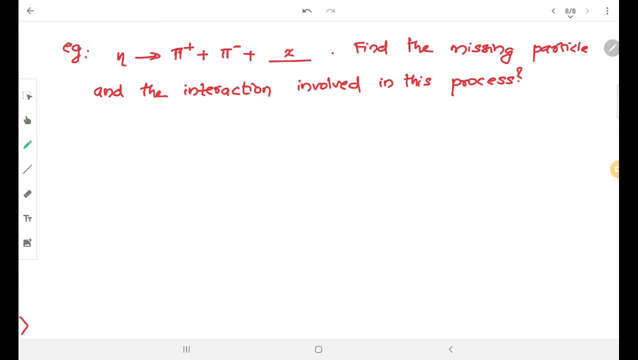 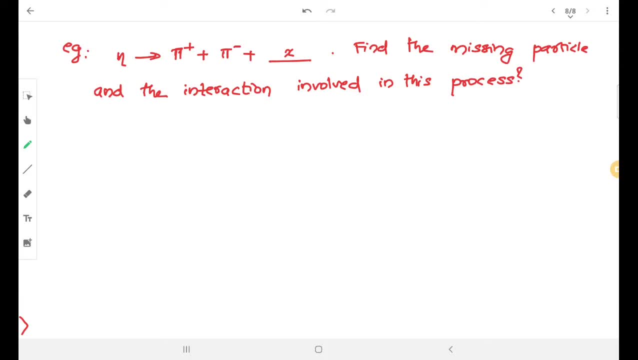 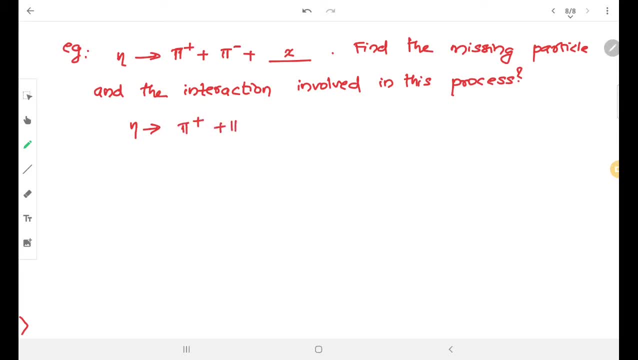 Eta gives Pi plus IZ. Let us write: eta gives pi plus plus, pi minus plus x. So first let us look at charge conservation. We have to identify which particle is x. When we look at charge, eta's value is 0.. 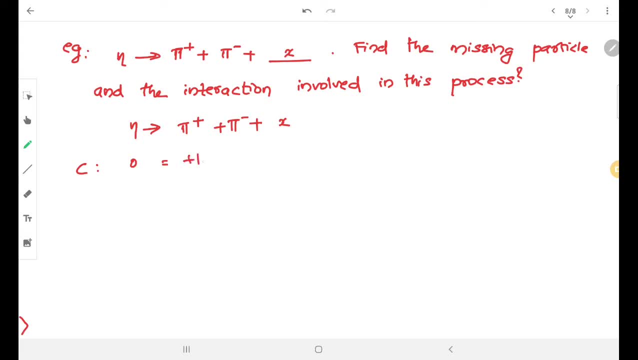 eta's value is 0, equal to pi plus plus 1 minus 1 plus x, So it should be a chargeless particle. So we have to conserve charge. Okay, Next let us look at spin. Spin is 0 for eta. 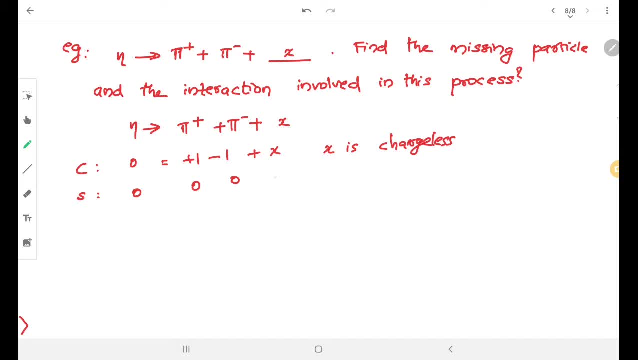 Pi plus is 0.. Pi minus is 0.. So x is spinless particle, x is spin equal to 0.. Next let us look at strangeness. Eta is not a strange particle. Pi plus is not a strange particle. 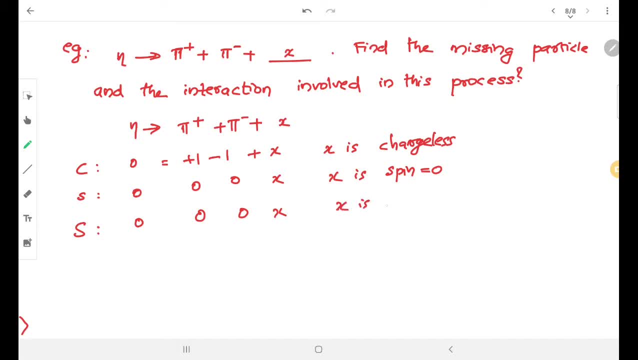 Pi minus is not a strange particle, So x is not a strange particle. Anyway, we have understood that there are no kaiyans and hybrids. Okay, Next, let us look at conservation of i. Let us look at conservation of i. 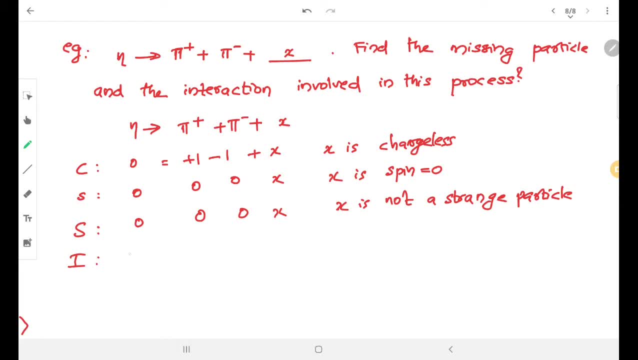 Eta has a value of what Eta is. a singlet Pi's value is 0.. Now pi plus. Pi plus has a value of 1.. Because it is a triplet, Pi minus has a value of 1.. 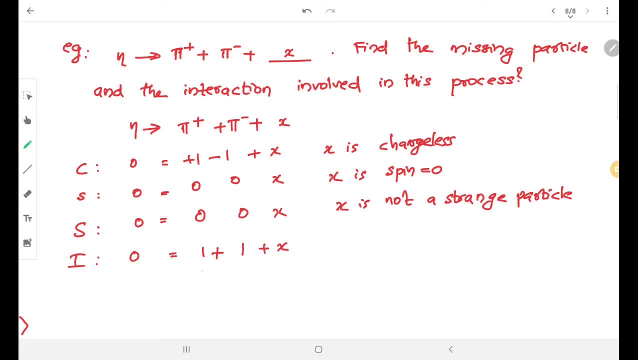 So what will be x? Okay, Spin addition here is not just summation. On the left side it is 0. So x is 1.. When we combine these 1 and 1 on the right side, what are the possible values? 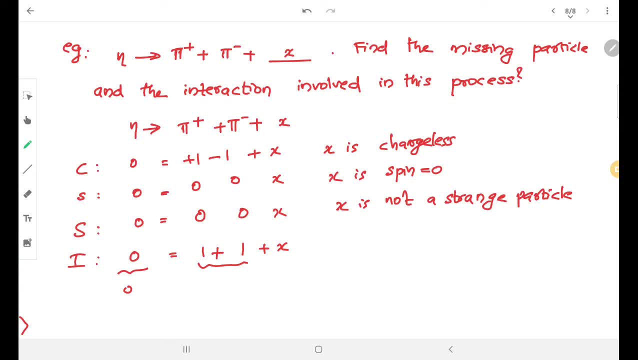 When we do 1 plus 1, the values will come from modulus of j minus 1 to modulus of j plus 1.. The values will come from modulus of j1 plus j2 to modulus of j1 minus j2.. Here, from 1 plus 1 to 1 minus 1, what are the possible values? 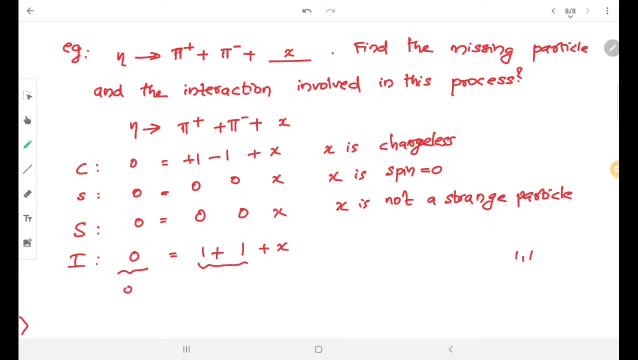 When the combination of 1 and 1 comes, when we add 1 and 1, the possible values will come from 1 plus 1 to 1 minus 1.. That is all the values from 2 to 0 are possible. 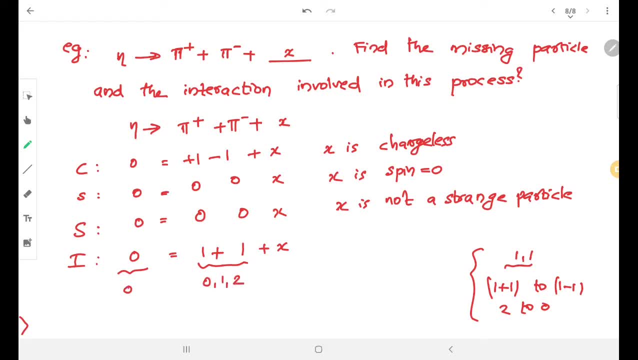 All these values are possible. If 0 on the left side has to come. what is the value of x If the value of x is 0, i will be conserved here. So what is the value of x? What can be the value of x? 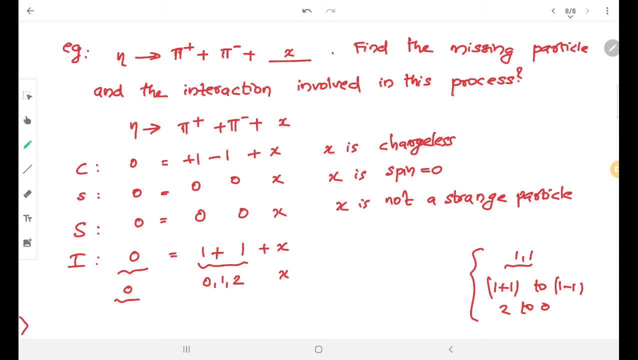 The value of x can be 0.. When we bring 0 and 0 together, 0 will come here. Now the value of x can also be 1. Because if the value of x is 0, there is 0 here. 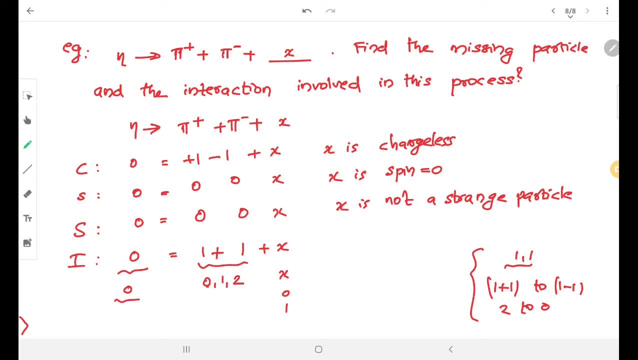 So 0 plus 0 gives 0. Now, even if x is 1, it is possible, Because in 1 plus 1, 3 values are possible. 2 to 0 is possible. So the isofin values that can come from x are 0 and 1.. 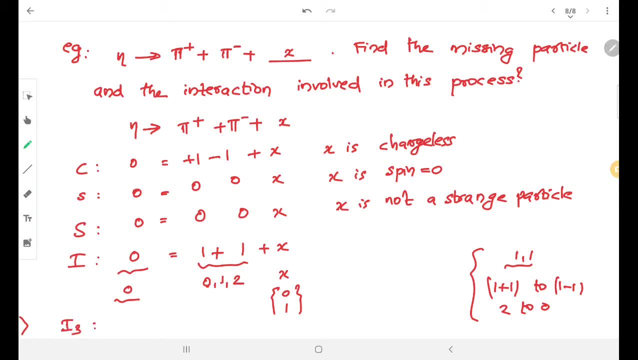 These are the possible values. Now let us look at i3.. Let us just add i3.. Before and after processes: if the sum of i3 values is same, it will be equal. Now the value of i3 is 0.. 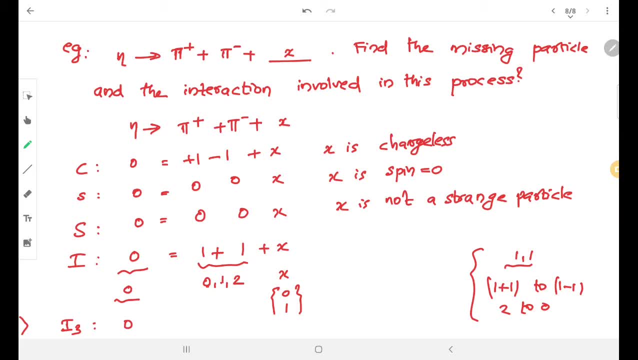 Because, since it is a singlet, the value of i is 0 and the value of i3 is 0.. For pi plus, the value of iz is plus 1.. For pi minus, the value of i3 is minus 1.. 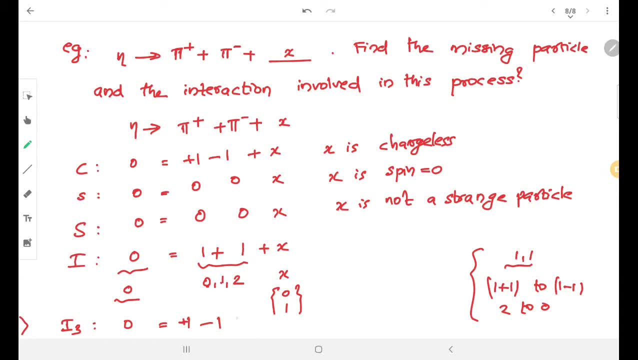 Okay, So i3 has to be conserved. For i3 to be conserved, the value of i set is 0.. The value of i set is 0.. The value of i set is 0.. It is a particle without charge. 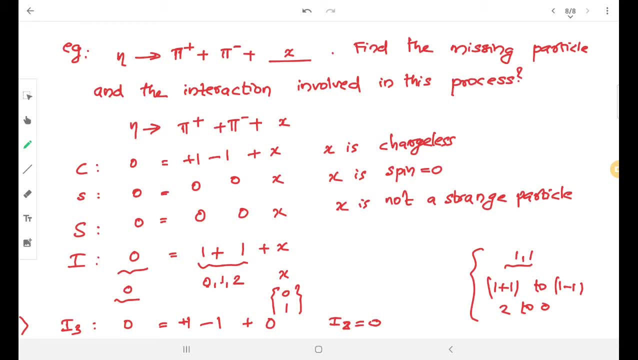 The spin is 0. It is not a strange particle. So it is not a strange particle. The Hadrons behind the particles using isosin form numbers, are pi ones. It will not be pi ones. So for pi ones pi will come as pi plus pi minus, pi zero. for pi ones family. 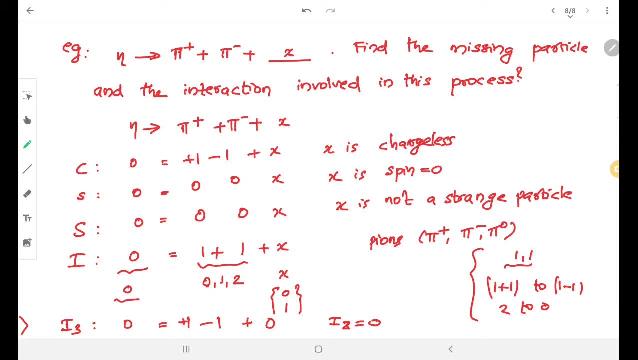 Okay, So pi plus and pi minus is a charge, So there is a particle left without charge, That is pi zero. The value of I0 to Iz is 0 and the value of I is 1.. We said that even if the value of I is 1, this reaction is possible. 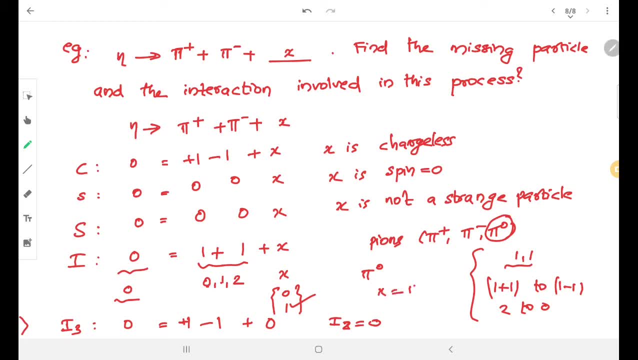 Here. what does x mean? x is equal to I0.. The missing particle is I0.. Is eta 0 possible? You might be wondering. If the value of I is 0 and the value of Iz is 0, then eta is 0. 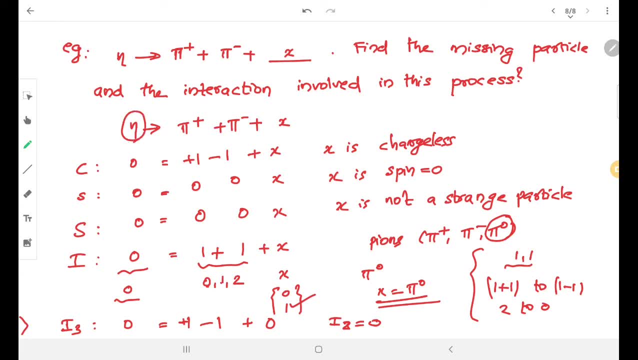 But eta actually decays. If eta decays, then eta will not come. So the only possible particle in this is a neutral pion. Here I and I3 are conserved in one interaction. Here I and I3 are conserved. 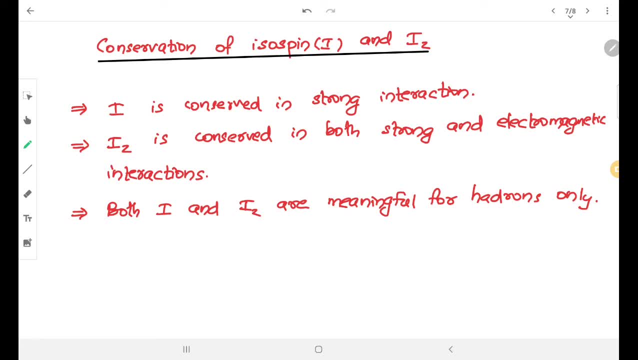 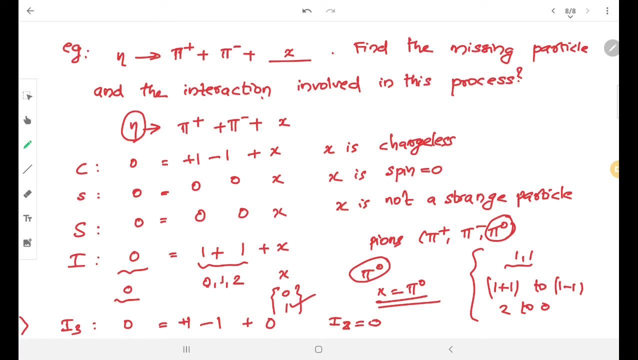 We saw earlier that I is conserved in a strong interaction and Iz is conserved. So the two possibilities are strong and electromagnetic, But I is conserved only in one strong interaction. So what is the interaction involved in this process? 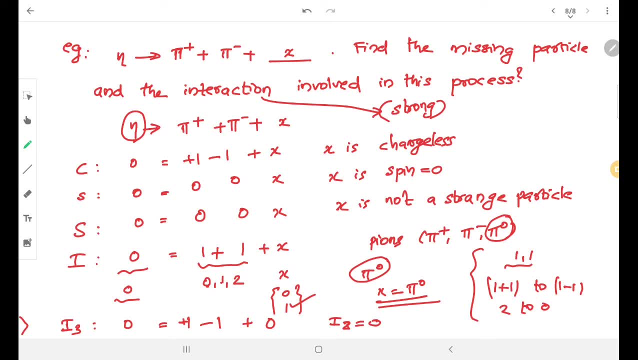 It is the strong interaction. So we have found the missing particles. Now we know which interaction is involved in this process. In this way, we can find the missing particles, Which are the missing particles we will need now in thisеляing esse. 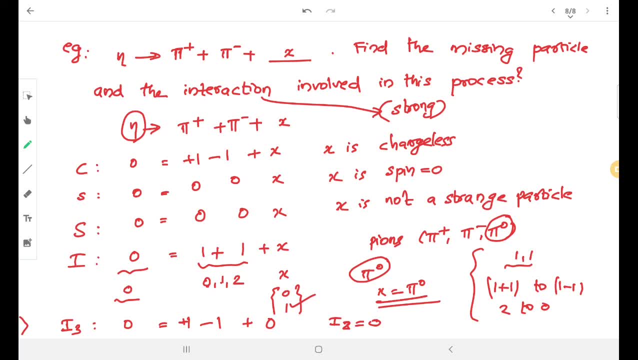 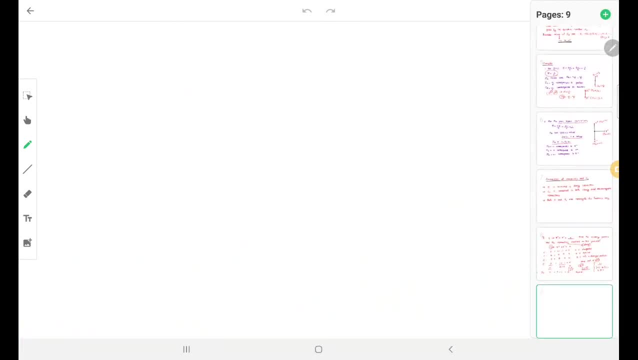 Now this is the problem in your university examination. Let us talk on what is conservation loss involved in this problem? This is considered as the missing particle. We have temperature mu is present in this problem. X on a missing particle. Find X, Find X. Ok.